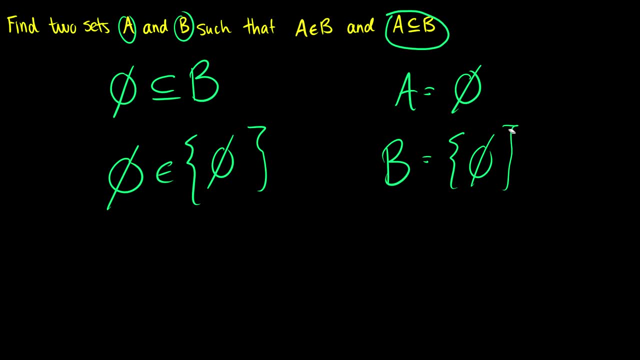 as the set containing the empty set, And now we have sets A and B, such that A is an element of B and A is a subset of B. So whenever you see these weird conditions where you have both an element and subset, the first thing you should always consider is the empty set and you should consider: 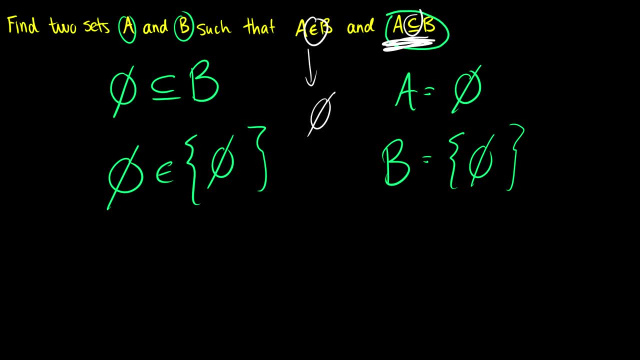 some properties related to the subset, like what holds for everything. Is there something that is an element of every set and what holds for every set? So we're going to look at that, and we're going to look at the set that contains the empty set, and we're going to look at the set that contains the. 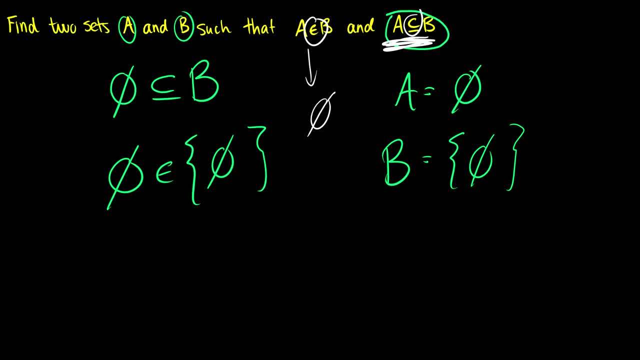 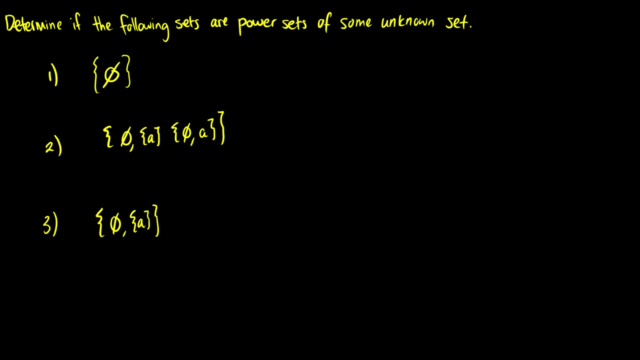 empty set and the answer is no, But there is something that is an element or that is a subset of every set, and that would be the empty set itself. So you can construct your sets like this, Okay. second question: Determine if the following sets are power sets of some unknown set. 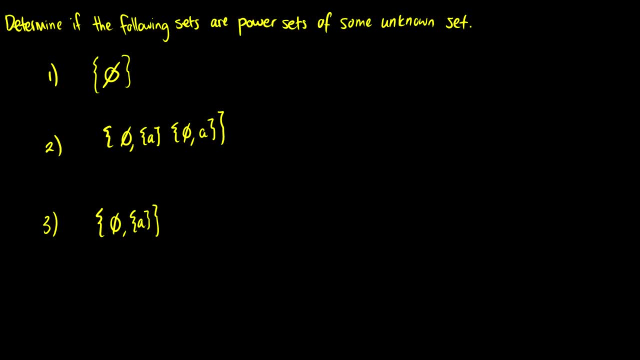 So what I'm saying is: okay, I'm giving you a power set or I'm giving you a set that looks like a power set. You have to tell me if it is a power set or not. So first question: We have the set containing the empty set, So this has two to the zero elements, just equal to one. 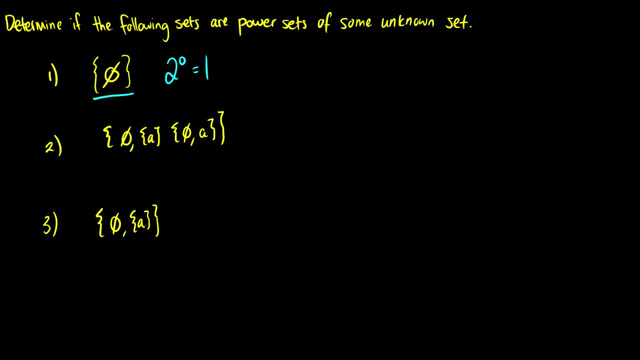 So this is potentially a power set. So what can it be the power set of? Well, what about the power set of the empty set? Okay, what is the power set of the empty set? Well, it's the set containing the empty set, and that's exactly what this is. 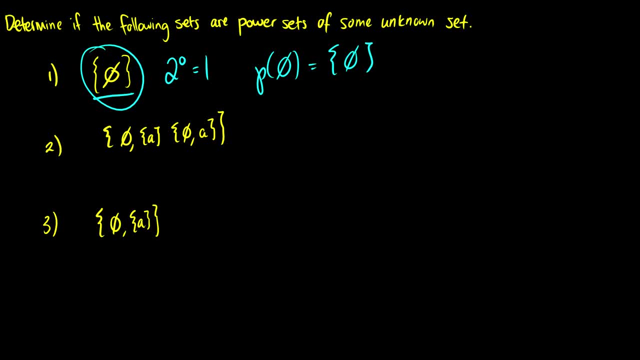 So of course, the first one is a power set. So that's the power set. Three, two one and weakened Okay. okay, so to do that you need to find two sets. So there's three, if we want to get just a last set. 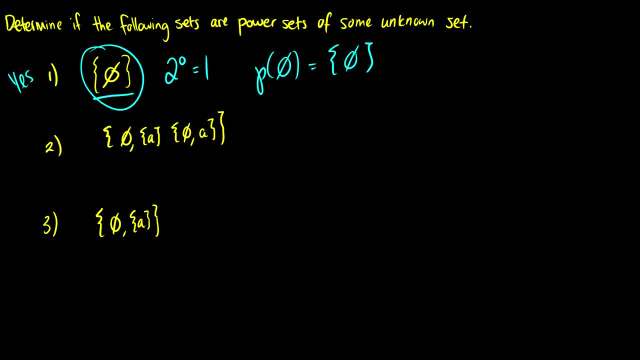 set, mainly of the empty set. okay, number two: we have the set containing the empty set, the set containing a and the set containing the empty set and the set containing a. so this has three elements in it and this is not equal to 2, to the power K for some K in our positive integers. so this is not going to be a.